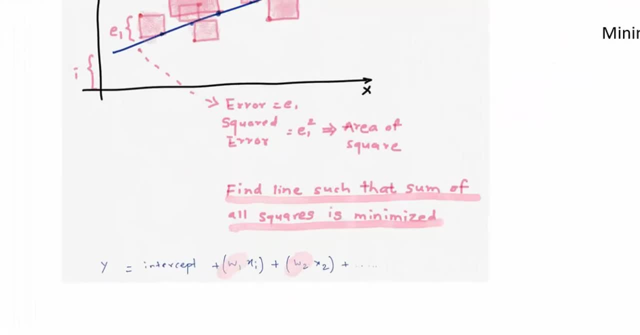 we say we want to get a linear model or linear regression. model is essentially we are calculating these weights. So you can think of linear regression as weighted sum of all the features. So y is our predictor variable, the target variable, and x1, x2 are our predictors and 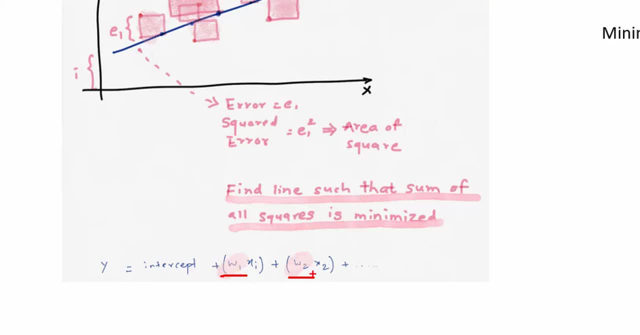 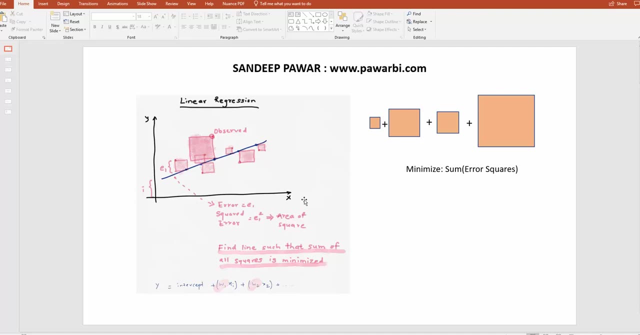 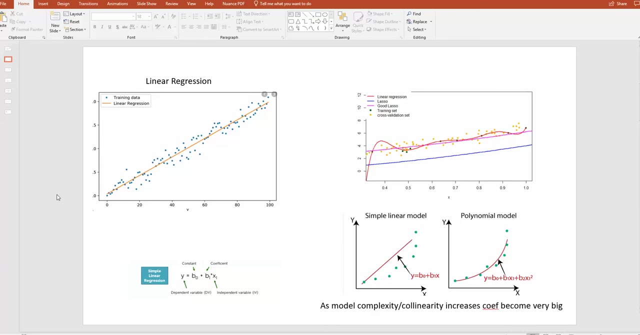 we want to find these weights to and then to sum them up so that we can predict y. So, again, all we are doing is find the minimizing the sum of these squares and find these weights. Now, linear regression is good, but, and again, why it's called linear regression is because of this additive factor. 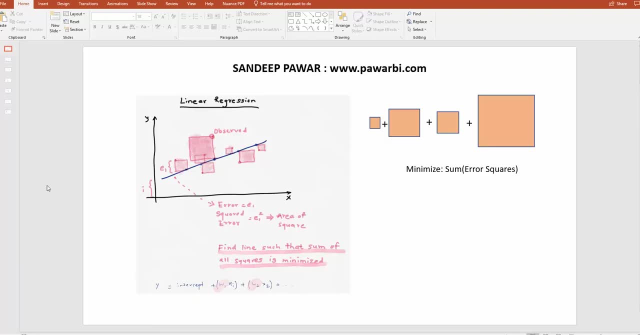 We are adding all these predictor variables together to predict our target variable. It is not because we don't have any power term with x or you know anything else. It could very well be, you know, w1 times sine of x or tan of x, and it will still work the same way. 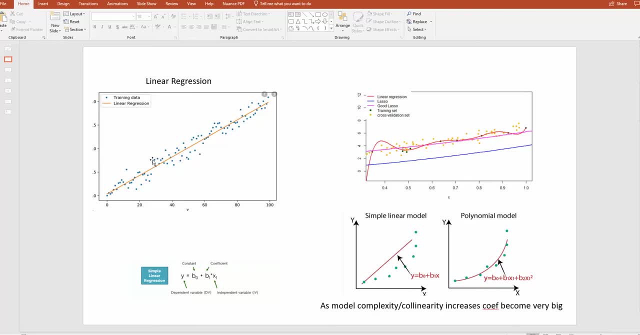 So the reason why linear regression is a problem is a couple of things. First, in linear regression, we assume that all our predictor variables or features are uncorrelated with each other. So that's the reason why linear regression is a problem is a couple of things. First, in linear regression, we assume that all our predictor variables or features are uncorrelated with each other. 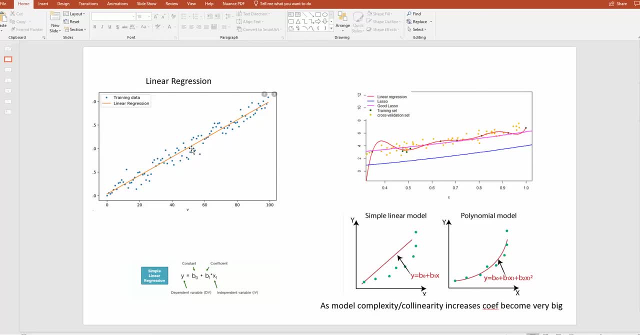 If they are correlated with each other, then what happens is these factors or these weights, w1, w2 or, on this slide, I'm calling them as B, but these become inflated, they become very large and if, as the model complexity increases, so, as I show over here, we could create a more complex model. 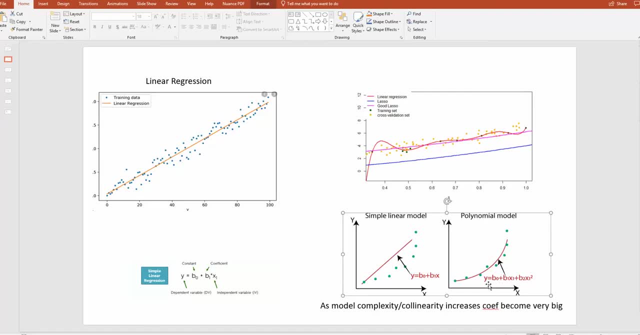 to fit our data. so in this example we have: y is equal to b naught plus b1 times x1 plus b2 times x1 square. so clearly there is a quadratic relationship here and we can capture that by using linear regression but using higher polynomial or term. so we are just getting the square of the x1 term. 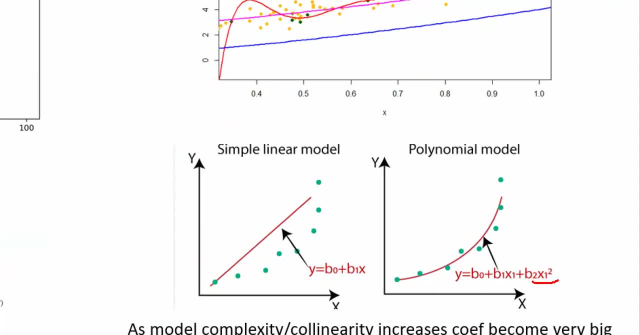 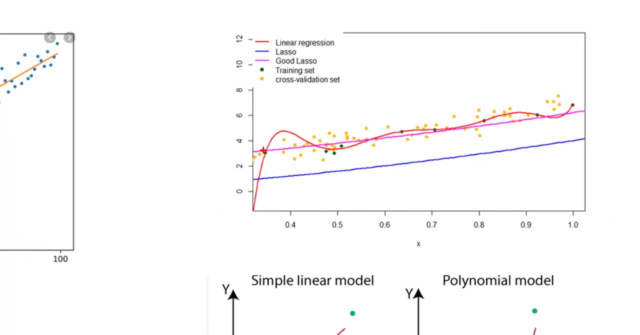 here, x1 term over here and again. this is not a well. this is still linear regression, because we are adding all the terms together as we start adding these polynomial terms, as you can see over here. if this was our linear fit over here, then this red line, this wiggly red line, is our. 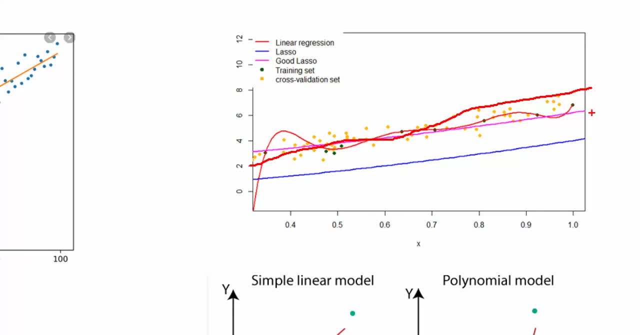 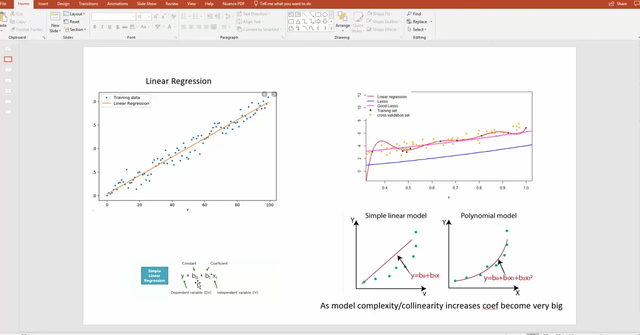 polynomial fit and as we start increasing the order for order of our polynomial, the model becomes more complex, and the way to identify if a model is complex is to keep an eye on these weights. so when the model has high bias and it is very simple, these weights are rather small. but as you start adding more polynomials, 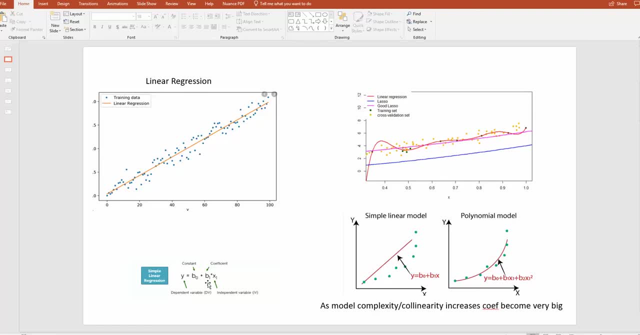 or even you have multi-collinearity, these weights become very, very high and- And that's how we define complexity, or that's how we can track complexity- In case of linear regression, the way we can get around that is penalizing these weights. 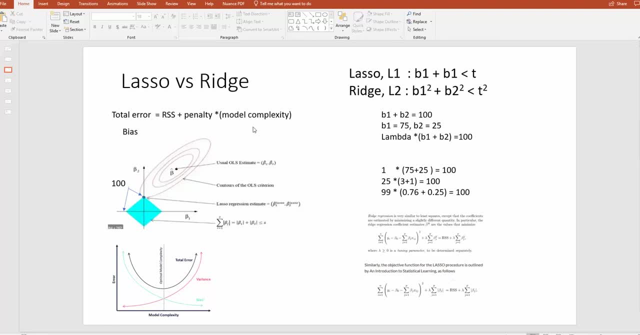 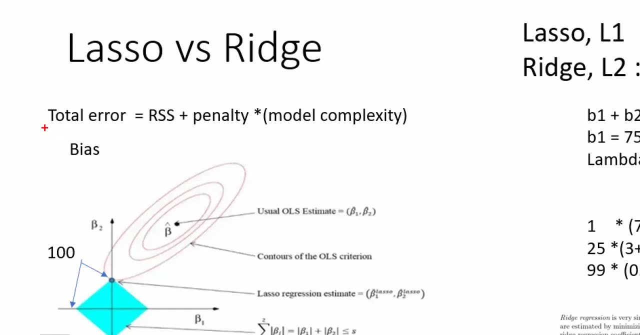 And the way we do that is using lasso and ridge regression. So again, in case of linear regression, we have the total error. mean squared error is root sum of square, which is again all those squares that we earlier talked about. 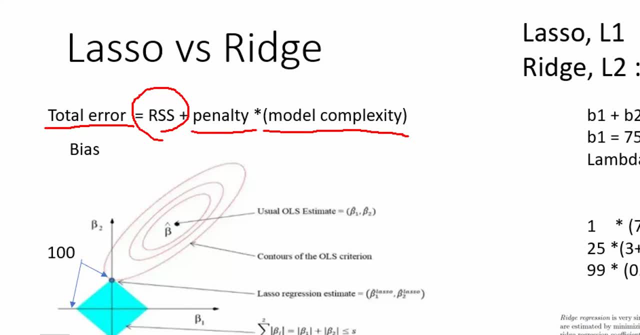 And then model complexity multiplied by penalties. All we are saying here is that we want to penalize or regularize this model complexity. And this model complexity, as I said earlier, is tracked by how high those weights or the coefficients become, And there are two ways to do that. 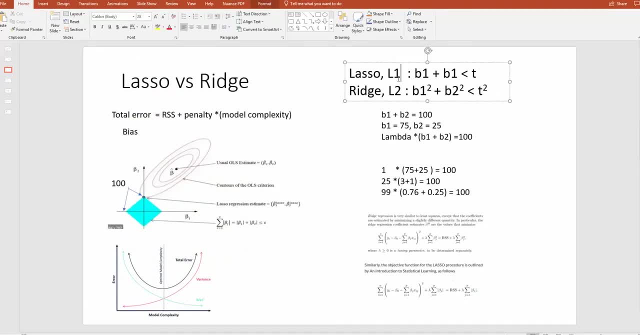 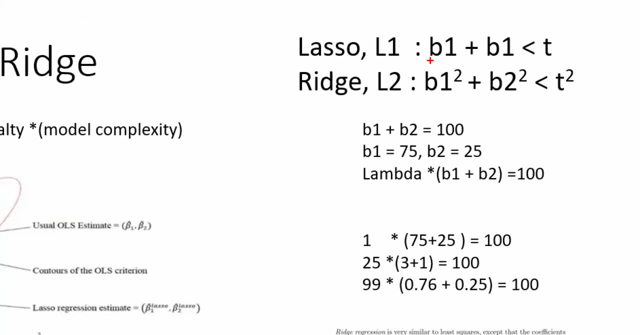 One is if we use lasso regression or ridge regression. In case of lasso regression, these weights the w1 or the b1 that we talked about earlier. we just sum them up, And if that number is very high then we know it's a complex model. 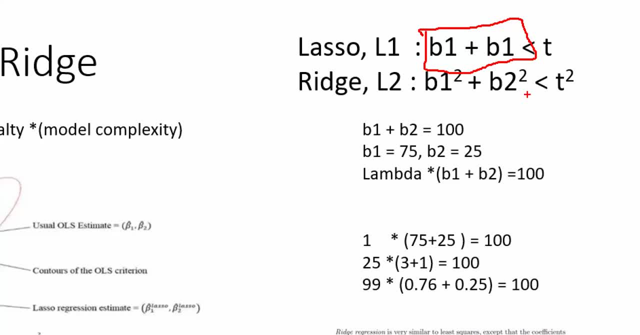 In case of ridge regression, however, we square these terms, all of these terms, and then calculate the complexity. And in case of ridge regression, however, we square these terms, all of these terms, and then calculate the complexity. LAUGHTER: 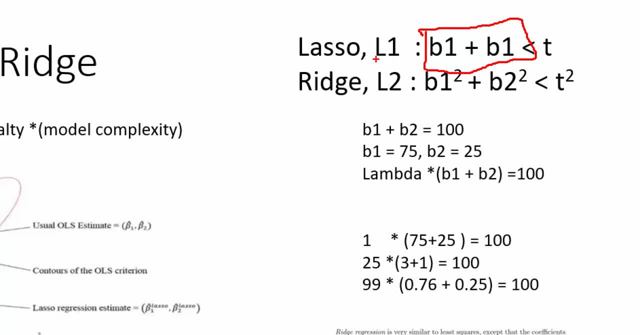 Mathematically speaking or statistically speaking, if we just use order one, then it's l1 penalty, And if we use two, it is l2 penalty. If we use three, then it's l3 penalty. It's just a norm of a vector. 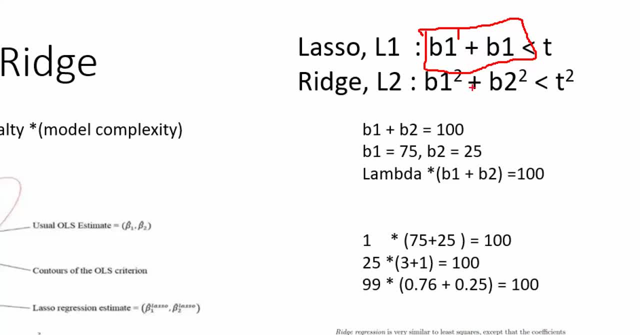 So one or two are called norms and it's just the norm of a vector And the way it works in penalizing is. I can give you an example. Let's assume we have these b1 and b2.. this b1 and b2, and we start off with b1 plus b2 is equal to 100 and b1 is 75 and b2 is 25. 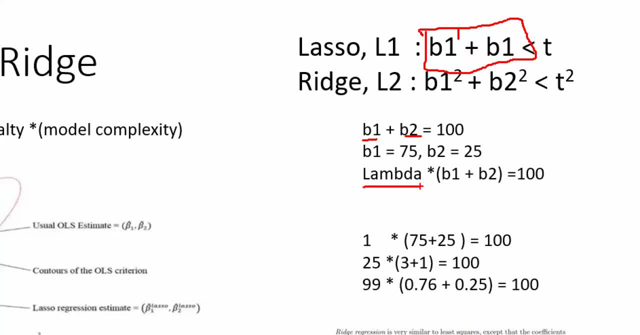 then we add this lambda term, lambda being our penalty term times b1 plus b2 is equal to 100, is our new equation. if i choose this: lambda is equal to 1, then it's 1 times 75 plus 25, 100. if i do increase that penalty on lambda to be 25 now to keep this number 100 the same, 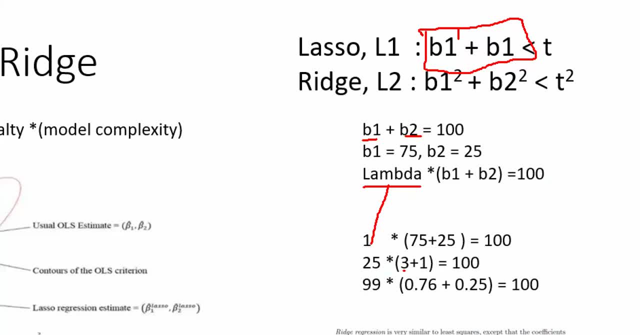 the weights will have to go down. so now the new weight is 3 and 1. if i increase it even further, the penalty is now 99 and to keep the number the same, 100. remember we are trying to minimize all of this at the same time. so when i increase it to 99, the coefficient becomes 0.76 and 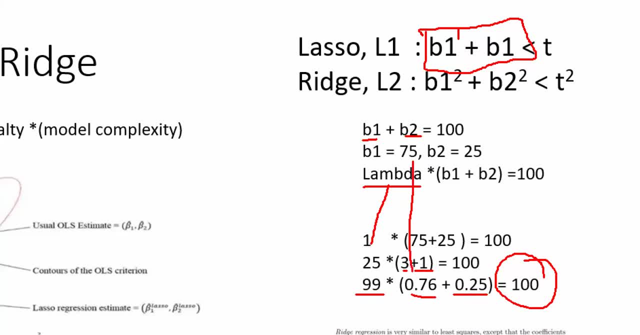 0.25, so it has now come down from 75 all the way down to 76 and 25 to 0.25, just as an example. so that's what we essentially, we are trying to do by increasing these, by assigning a lambda value. 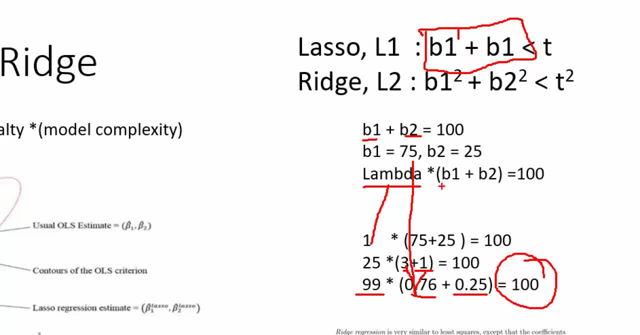 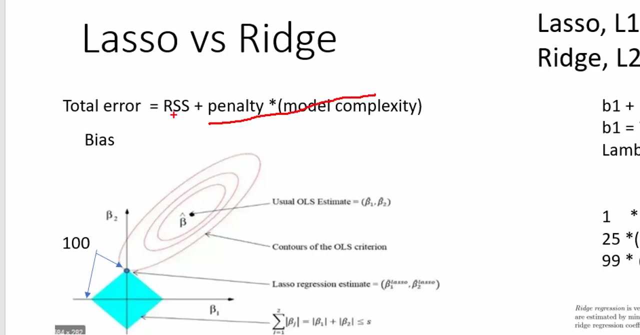 to these weights. we are trying to reduce the reduce these model by this model complexity, so as the lambda value: when the lambda value is 0, then if we come back over here, if the lambda value is 0, then this whole term goes away and then we just have RSS and RSS is are just a good old. 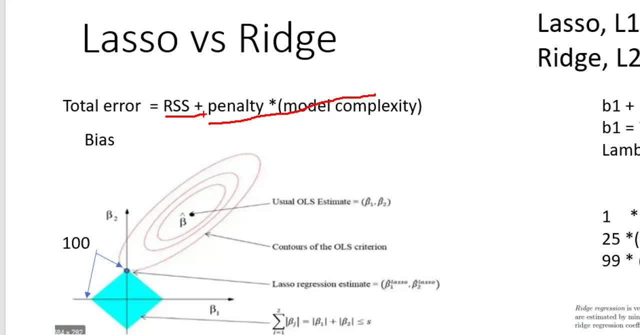 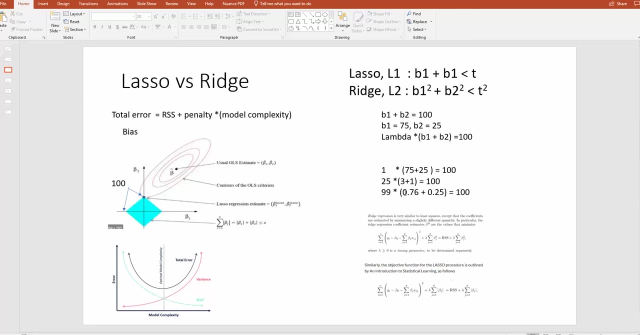 old linear, linear regression, or least squares aggression. so there's just, you know, our linear regression. there is nothing to it, but as we start increasing the penalty, as you can see, to compensate for the increase in the penalty and so as to minimize the whole cost function, these, these weights start to go down. now we can look at this visually. we can look at this: 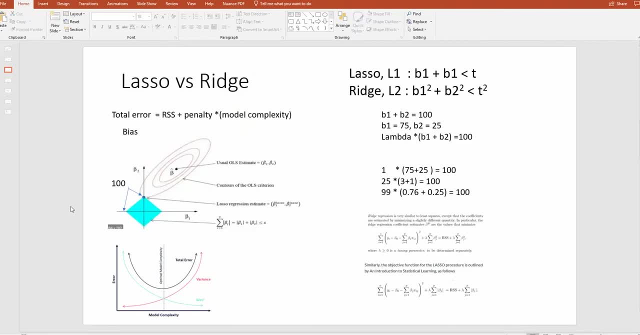 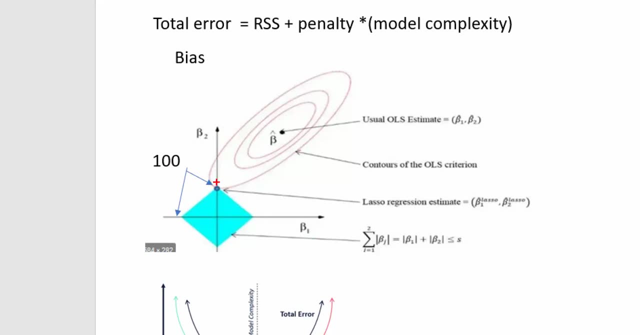 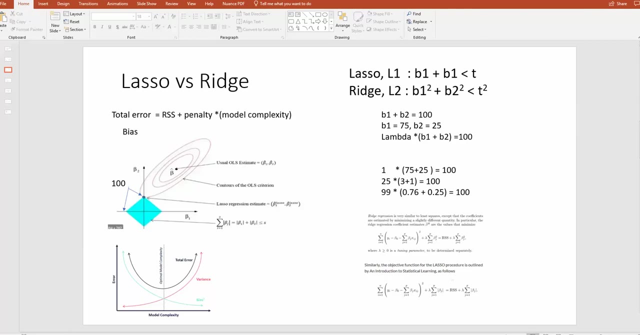 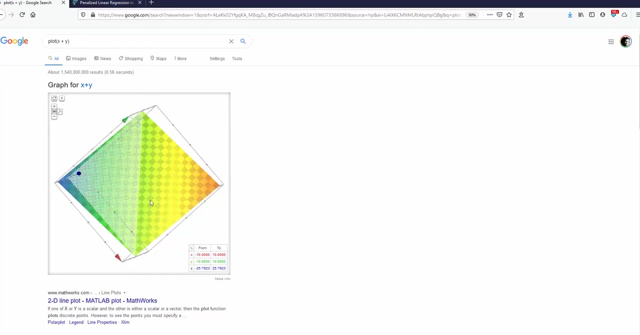 over here. so we have zoom in b1 plus b2 and if we plot b1 plus b2 we get this kite or diamond shape. this diamond shape is called an error surface. so if i go to google, for example, and just say plot x plus y, this is in 3D. but if we look down, because z is 0, you'll see we get. 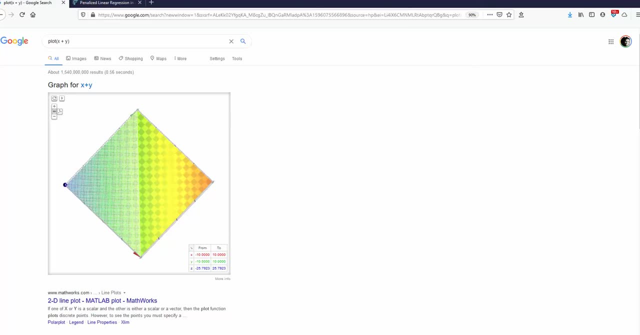 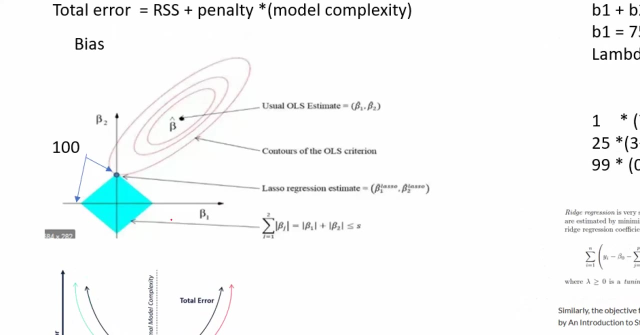 the diamond. so this is our error surface. so this diamond is nothing but this X plus Y that we have over here, so on, and we are considering only two dimensions. so we have b1, so feature 1 has a weight of beta 1, feature 2 has beta 2 and 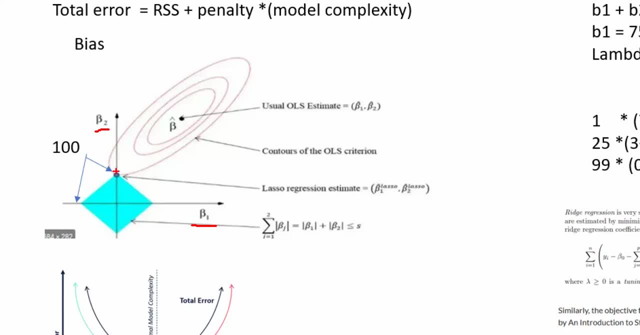 this is these vertices, these are. this is nothing but the hundred that we talked about earlier. this beta is our lasso, or rather the OLS, just the linear error, it's just the weighted coefficient from the linear regression that we have. now, as we start adding the penalty, we saw that the beta values, or these weights, 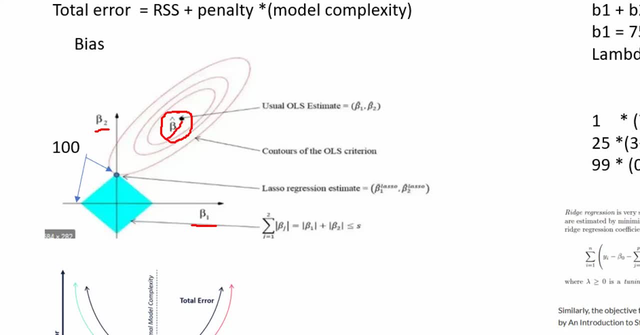 start going down and it keeps on increasing, keeps on increasing, increasing, increasing, increasing, increasing, until this constraint surface, or the error surface, or the error envelope, as they call it, it approaches that and it touches these. this vertices again, remember, this has to be hundred, so it can only be hundred if it either touches: 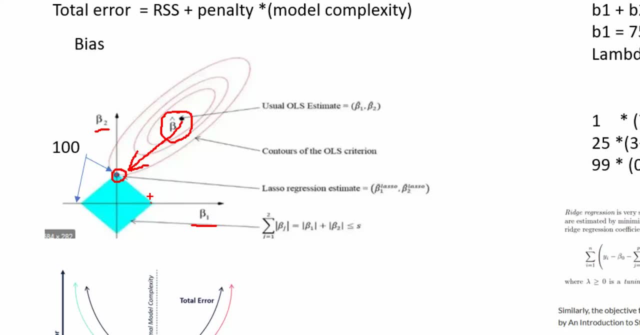 this point over here, or it touches this point over here and now what happens when it touches over here? beta 2 is hundred and beta 1 becomes zero at this point, or if it increases in such a way that it touches this vertex first, then beta 1 is 0 and beta 2, beta 1 is hundred and beta. 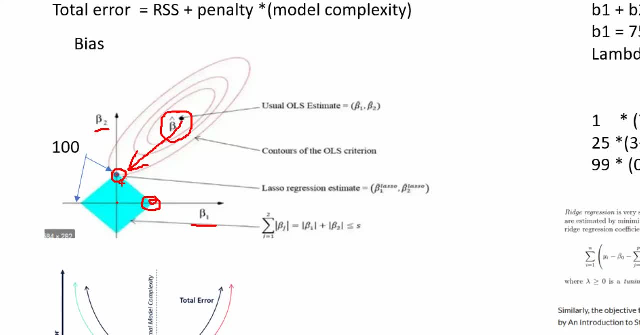 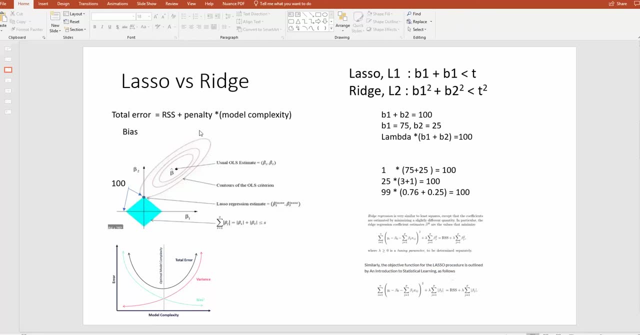 2 is 0, so that's how this works, and what happens when we are doing all of this is, as you can see, RSS is again our linear regression error. from the linear regression we are adding some penalty and we are adding more to the weight. so if we 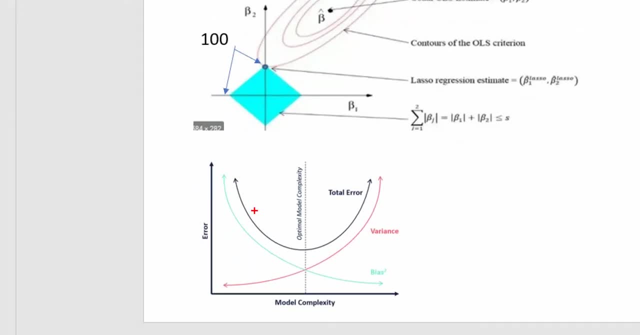 consider it in terms of buy-in's variance trade-off. as we add the penalty, our bias starts, the bias increases and but at the same time our model complexity starts to go down. so model complexity is now going down and which means our variance is decreasing, and then after a certain point we don't. 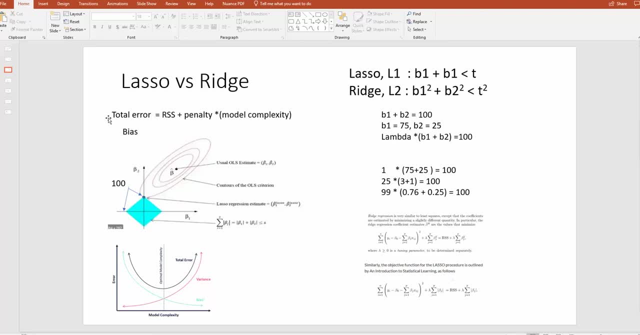 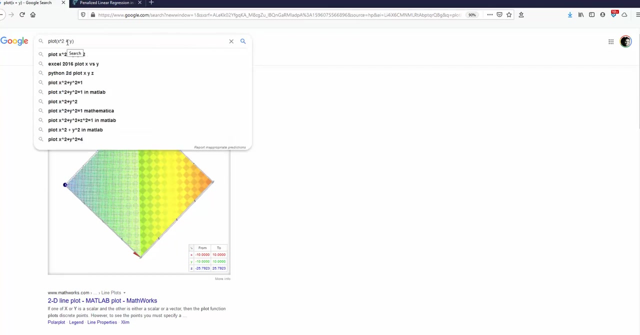 get anything more out of it. so the whole point of doing this is to increase the bias and then reduce the variance for as much as we can. then what happens in case of ridge regression? for ridge regression we are using the L2 penalty again. if we go back to our plot over here and then do X square and over here. 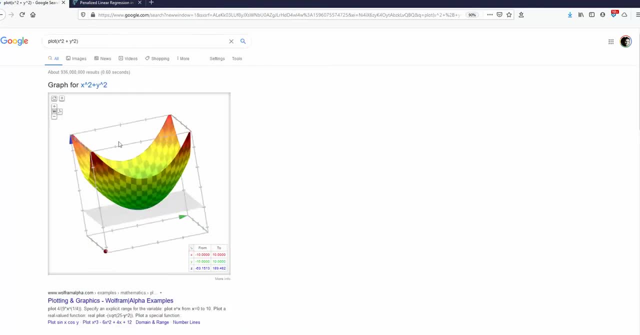 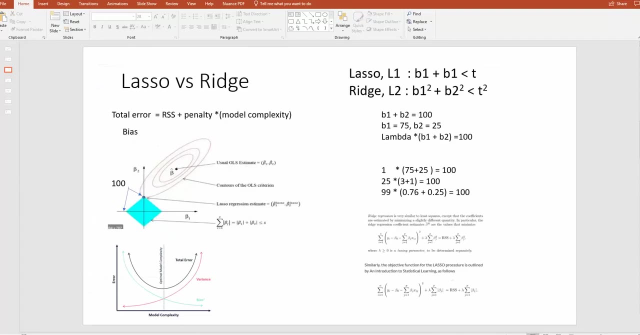 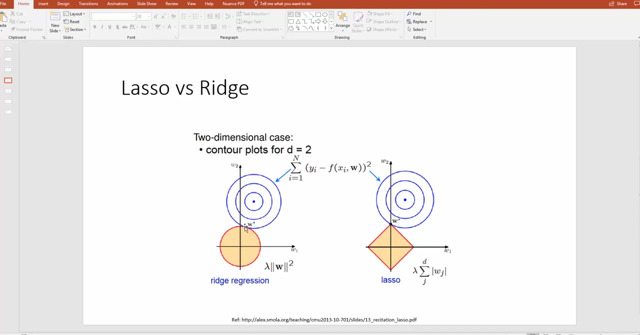 to square. this is nothing but an equation of a circle. so this is in 3d, that's why you see it like this. but if you look down you will see a circle. so our error surface in case of ridge regression is ridge regression is a circle. now we discussed the scenario. 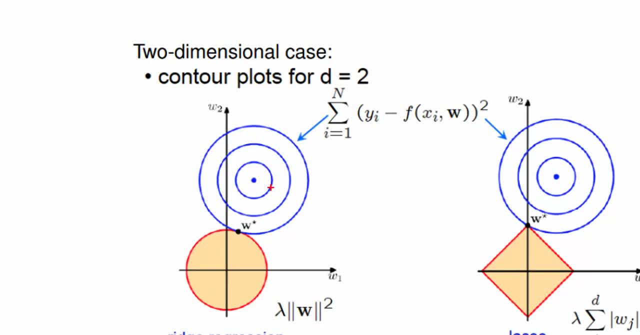 when, or we start penalising these weights. so as it increases- now again we are looking for this error surface over here, right, so as it increases, it does not. actually it may touch this vertex, but it is highly likely that it will touch this surface first, the here or here, and in that case the beta1 and beta2 are non zero, so in 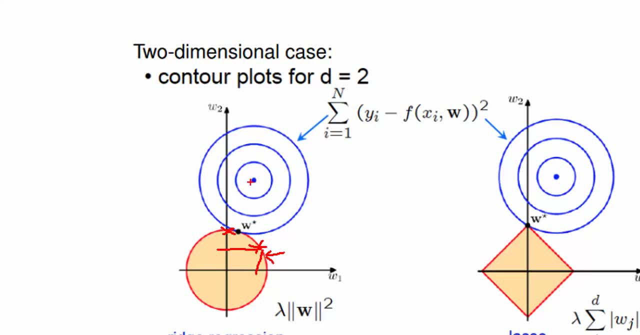 goes down from you know it was somewhere over here and then it has shrunk. so that's why it's called a shrinking mechanism. it has shrunk down from you know somewhere over here to all the way down to this value over here. so in case of ridge regression, we don't necessarily go all the way down to zero. it can go. 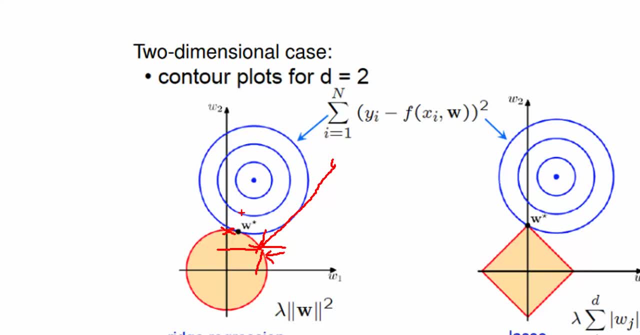 down to zero if we, if this contour surface expands in a way that it touches over here, but it's more likely that it will touch, you know, any anywhere else other than these four points. if it does add those four points, then the other weight will go down to zero or shrink to zero. so the benefit of using lasso 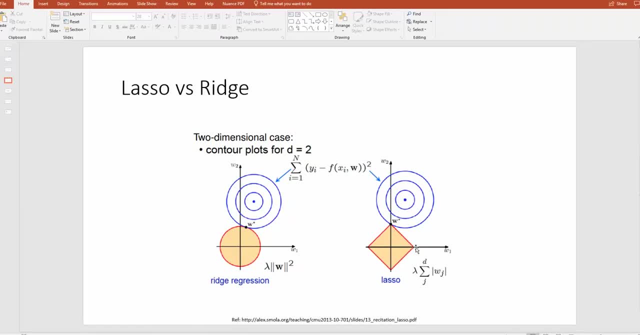 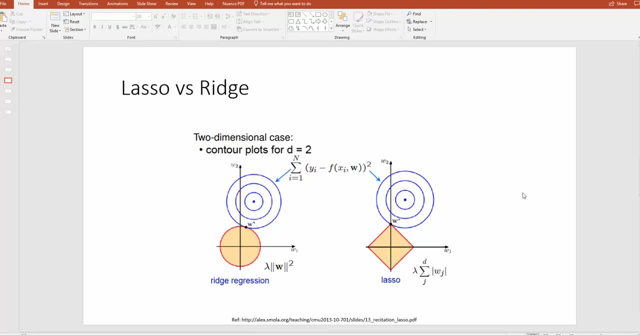 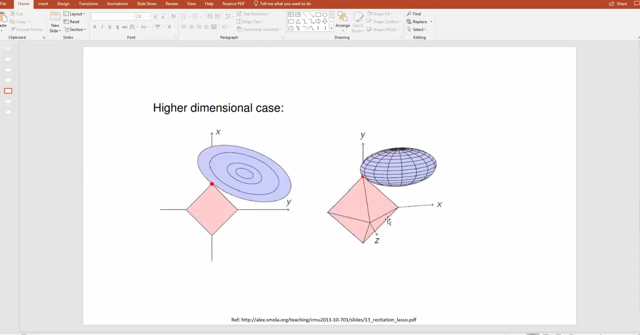 zero. so it can. that can be used for feature selection purposes, whereas in case of ridge regression they shrink down significantly but they don't necessarily go down all the way to zero. they may, but they will likely just shrink down by quite a bit now in higher dimension. so if we 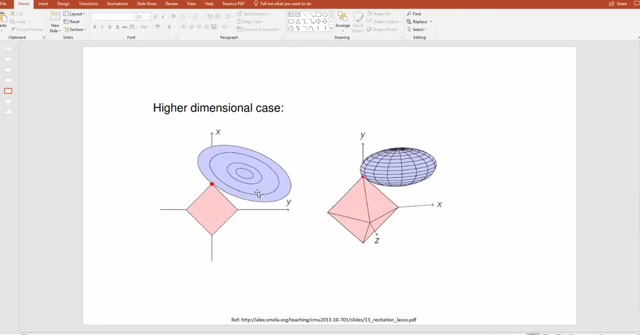 had three variables or three features: that diamond becomes or rhombus, so it works the same way, it starts increasing. and that diamond becomes or rhombus, so it works the same way, it starts increasing, then it touches the Vortex and then, when it does that, that particular 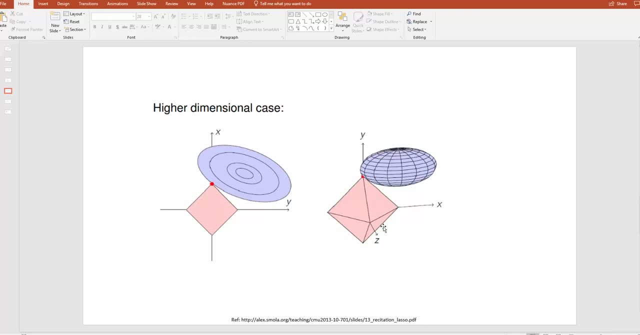 variable becomes one or hundred and the other two becomes zero, depending on wherever we touch it, but this would be in higher dimension. this would be much more complex than this if we use higher norm, so a norm beingubers and that we talk about inнитеam. 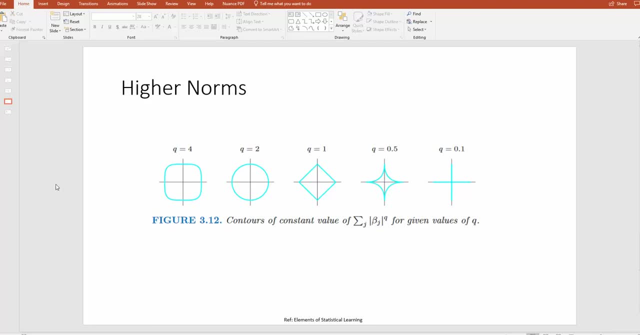 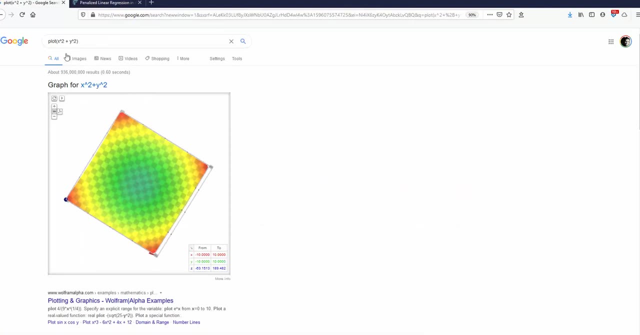 a norm being this L1 and L2 that we talked about in there. yes, and also if we target higher than 0, even so the value is not HTML threats. even so the value is not HTML threats about. I'm so if we use the higher norm, Q, raised to 4, so if we go here and then 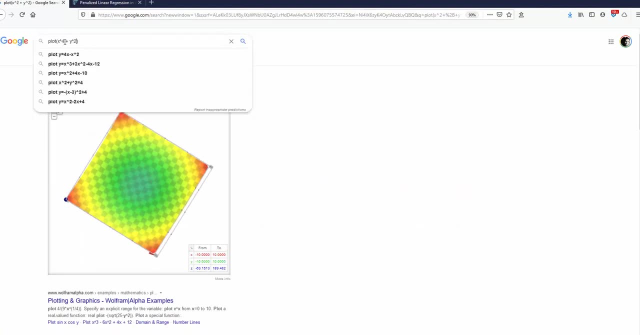 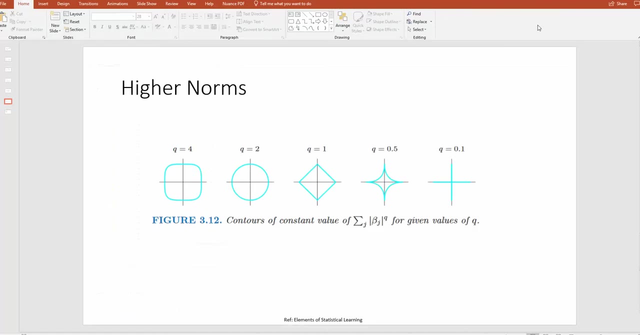 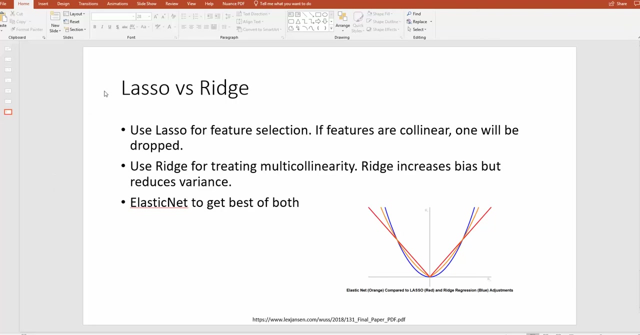 change it to 4, the this error surface starts becoming more funky. yeah, it's possible, but then it does not work. we don't get much by using higher norm. there are methods that use higher norms- Q thought norms- but that's really that's not very common. so that's what happens when we use linear regression with lasso. 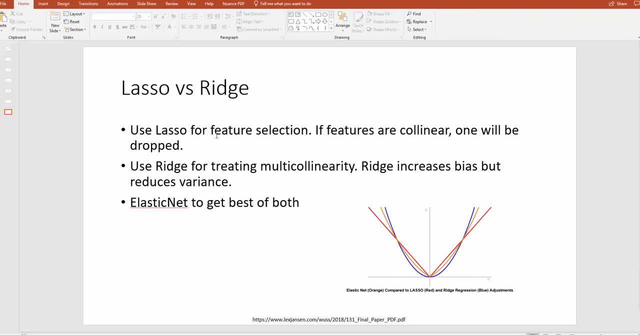 and rich. so the benefit of using lasso regression is feature selection and but if the features are collinear, lasso regression is a greedy algorithm so it will drop one of those features that that is collinear and there is no way to tell which one it will drop. so if you have X 1 and X 2, that are highly 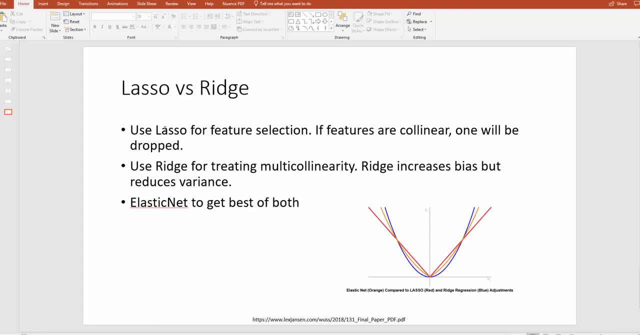 collinear with each other. in one iteration it might drop X 1, in the other iteration it will drop X 2, doesn't matter which, anyway other, because anyway it's, the two features are collinear with each other, so it doesn't really matter which one we pick. but just keep that in mind, that it's a greedy algorithm, so it 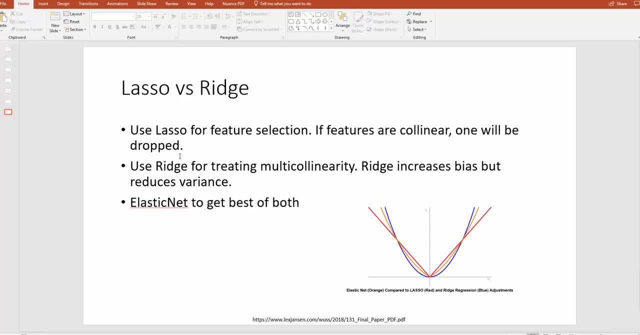 will drop. you know one of the two. in case of lasso rich regression, these multicollinearity is treated. you know one of the two. in case of lasso rich regression, these multicollinearity is treated by the rather than feature selection, so the features shrink down. but if you have 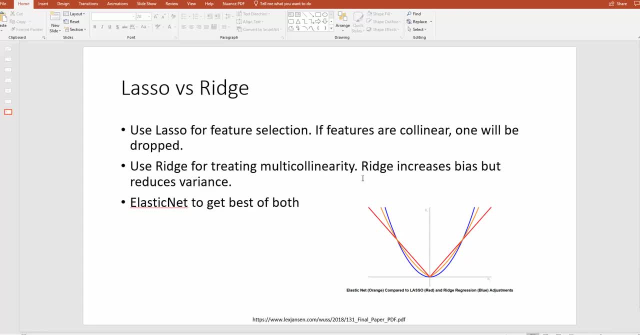 highly collinear features, then rich regression is used. and the way rich regression works is: if there are multicollinear features, then they will just shrink, but they don't necessarily go down to zero. and in case of rich regression we have higher bias but the variance goes down. if you want the best,